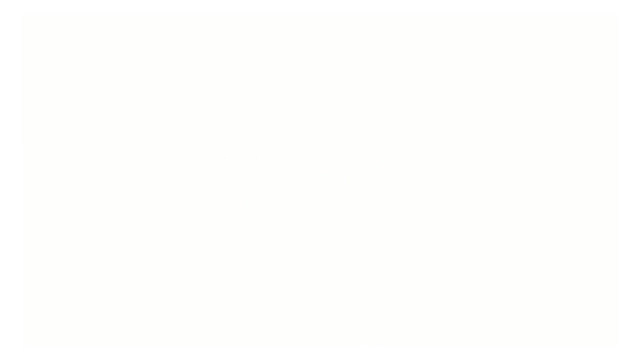 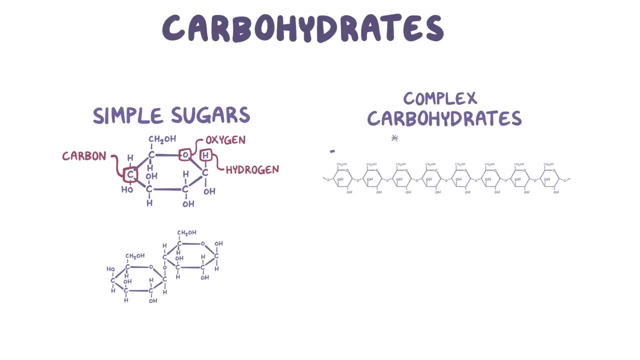 Carbohydrates include both simple sugars, which are little ring-shaped molecules made of carbon hydrogen and oxygen, either alone or in pairs, as well as more complex carbohydrates, which are formed when these rings link up together to make long chains Carbohydrates. 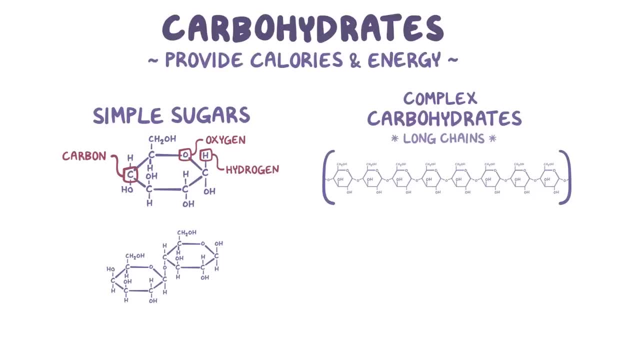 provide us with calories or energy, and simple sugars in particular play a lot of roles in our diet. They sweeten lemonade, balance out an acidic miso soup, fuel yeast in rising dough and alcohol, and help preserve jams and jellies. 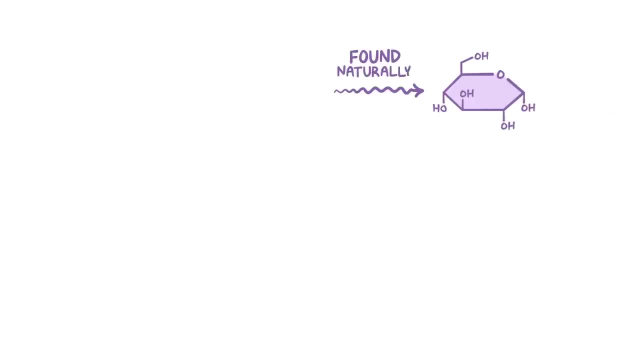 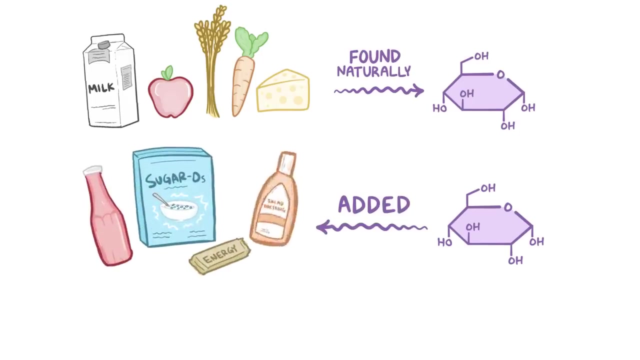 Now. sugars are found naturally in plants like fruits, vegetables and grains, as well as animal products like milk and cheese. Added sugars are the sugars that get added to foods like cereals, ketchup, energy bars and even salad dressings. 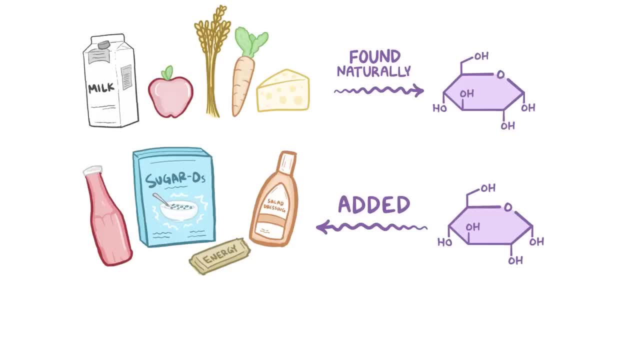 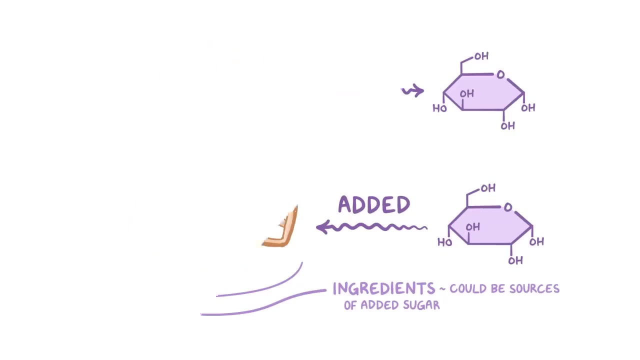 To be clear, even if the sugar being added comes from a natural source, like sugarcane or honey, it's still considered an added sugar. In fact, a variety of ingredients listed on food labels might be sources of added sugars, some of which you're probably familiar with. 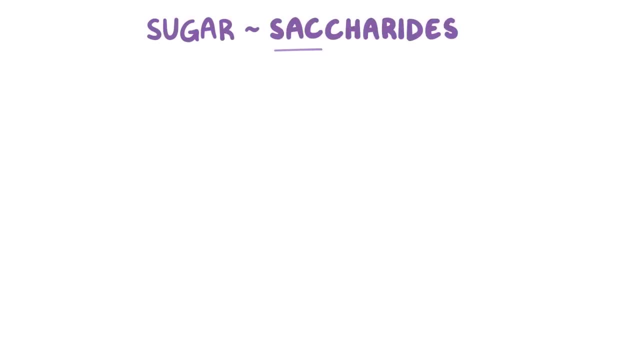 Sugar actually refers to a family of molecules called saccharides. Monosaccharides, where mono means one, so one sugar molecule. Disaccharides, where di means two and disaccharides, where di means two, So two sugar molecules linked together. Oligosaccharides, where oligo means a few, so it's three to 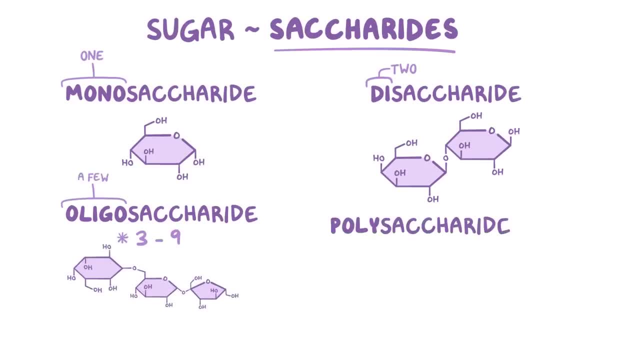 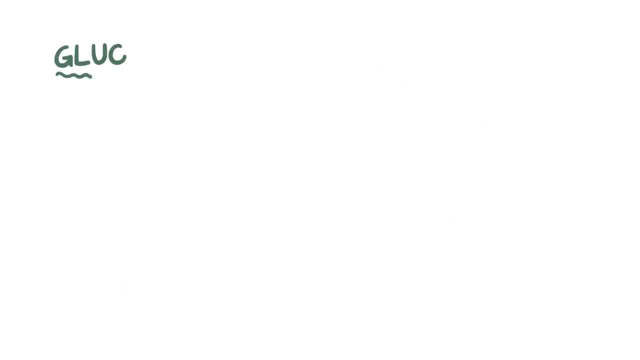 nine sugar molecules linked together And polysaccharides, where poly means many, so it's ten or more sugar molecules linked together. Glucose is the most important member of the sugar family and it's a monosaccharide. It's one of the main sources of calories for the body and is able to cross the blood-brain. 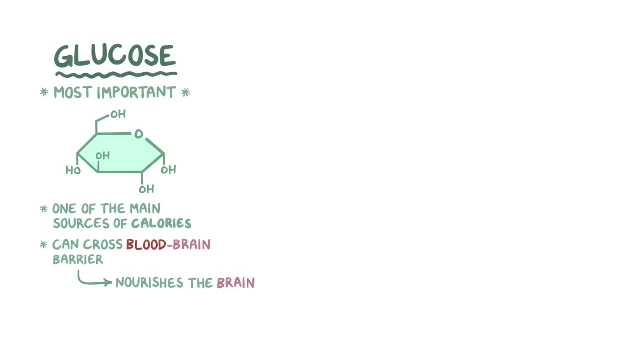 barrier and nourish the brain. Another monosaccharide is fructose, which is commonly found in honey, fruits and vegetables. Finally, there's the monosaccharide galactose, known as milk sugar. It's known as milk. 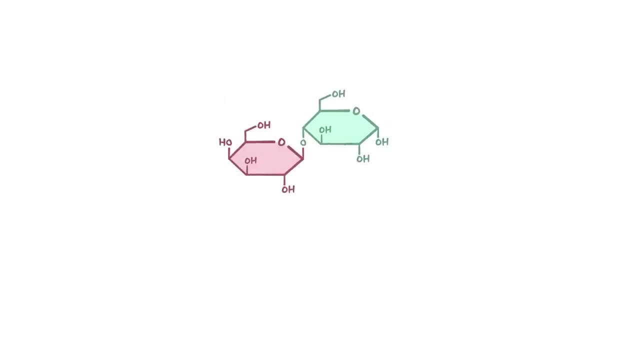 sugar because it's only found in nature when it links with glucose to form lactose, a disaccharide found in the milk of mammals, which includes cow milk as well as human breast milk. Sucrose or table sugar is another disaccharide, and it's formed when fructose is added to. 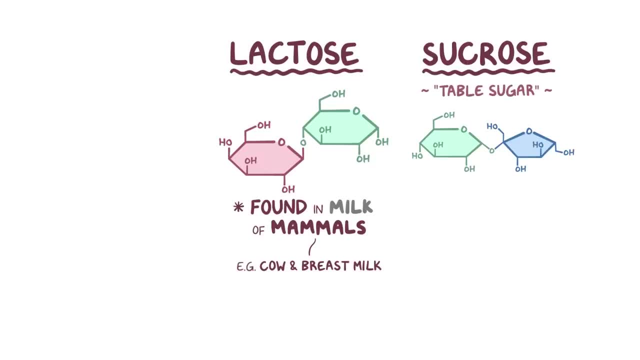 glucose Sucrose is found in various fruits and vegetables, with sugar cane and sugar beets having the highest quantities. Maltose is another disaccharide, and this one is two glucose molecules linked together, and it's found in molasses, which can be used as a substrate to ferment beer. 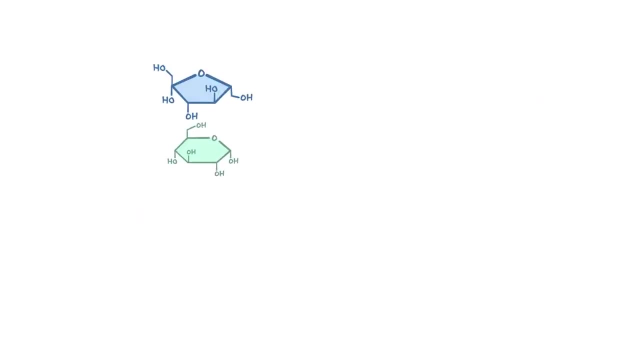 Sugars like fructose, for example, are most always found in combination with other sugars, and combinations can be pretty different, even in seemingly similar foods. For example, in honey, 50% of the sugar is fructose, 44% is glucose, 4% is galactose and 2% is maltose. 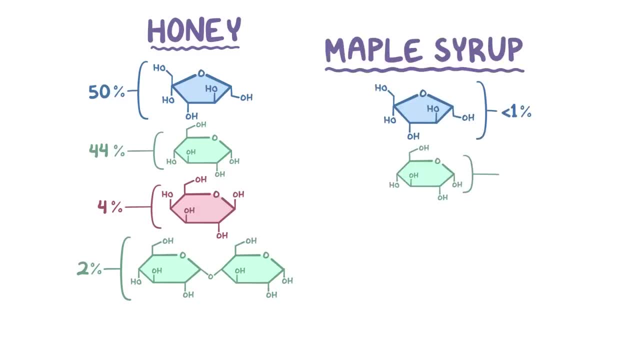 Worse in maple syrup, less than 1% of the sugar is fructose, 3% is glucose and 96% is sucrose. So simple sugars, whether they're natural or added, are mixtures of monosaccharides or 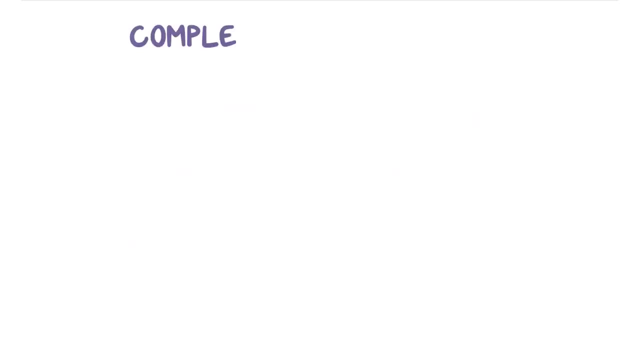 disaccharides. Next there are the complex carbohydrates. There are oligosaccharides like galactooligosaccharides, which are short chains of galactose molecules like those found in soybeans. Then there are polysaccharides, which are even larger chains. 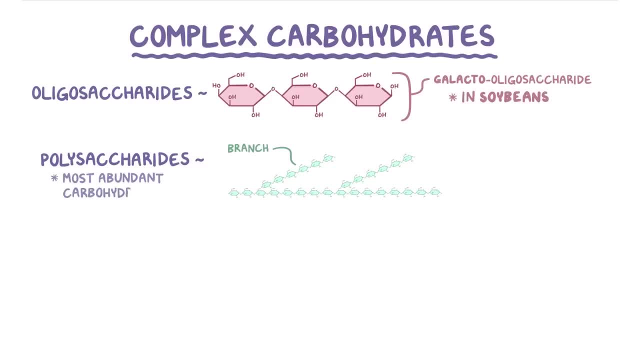 with branches and are the most abundant type of carbohydrates found in food. Starches are polysaccharides with molecular bonds between sugar molecules that human intestinal enzymes can break down. Starches are an important source of calories and can be found in foods like rice potatoes. 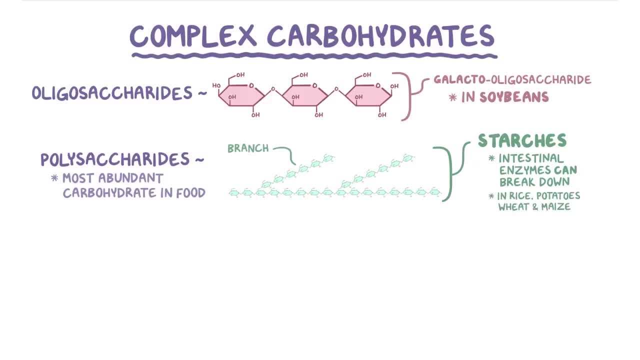 wheat and maize Starches don't taste sweet like simple sugars because they don't activate the taste buds in the same way. And there are also dietary fibers, which are carbohydrates that intestinal enzymes can't break down and so the body can't digest them. 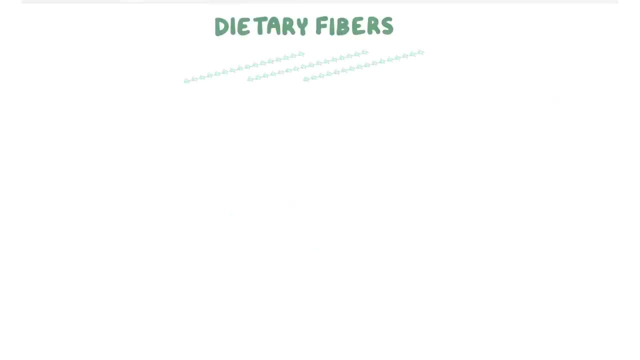 Now there are many different types of dietary fibers and they're not all the same when it comes to their structure or impact on health. Fibers have molecular bonds that are resistant to human intestinal enzymes, so they pass through the small intestine undigested, get broken down a bit by bacteria in the large. 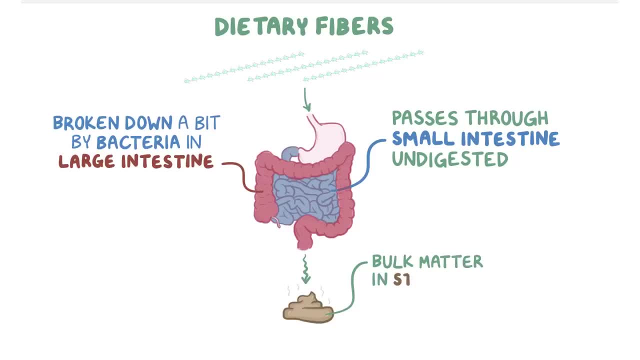 intestine and ultimately end up as bulk matter in the stool. Fibers are critical because they can slow down the rate of absorption of simple sugars like glucose in the small intestine, which can help maintain healthy blood glucose levels. They also increase stool weight, which can help maintain healthy blood glucose levels. 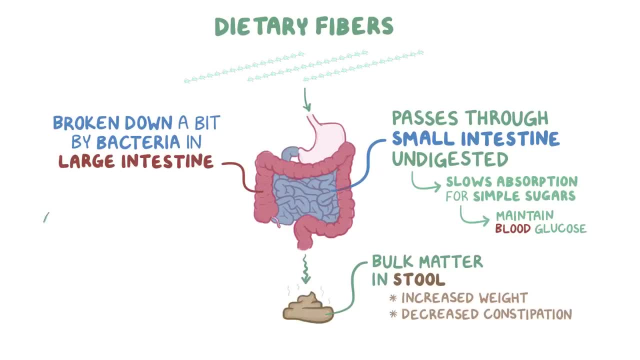 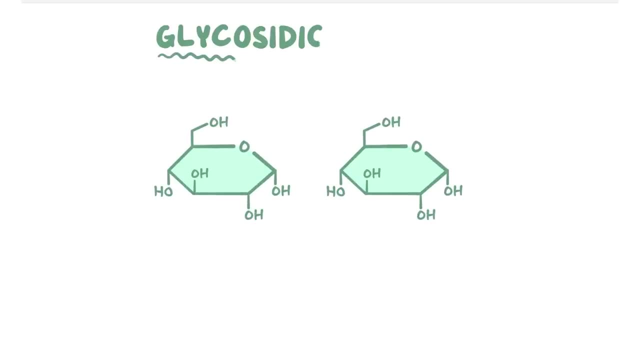 They also increase stool weight, which can help maintain healthy blood glucose levels. They also increase stool weight, which can help maintain healthy blood glucose levels. Monosaccharides link together through glycosidic bonding, which is when an OH group from the 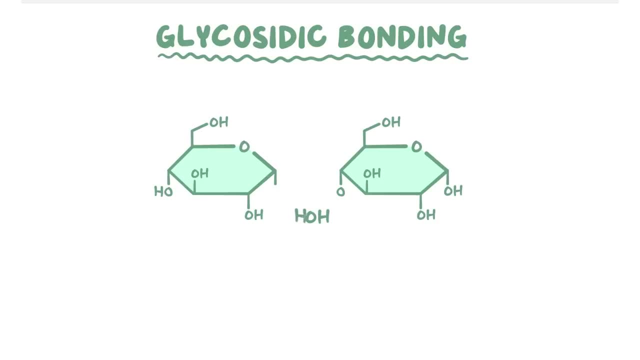 carbon on one monosaccharide binds with the hydrogen from the carbon of another monosaccharide. Together this forms an H2O or a water molecule, which goes away In the case of maltose. that leaves an alpha-1,4-glycosidic bond, which is a bond between carbon and glucose. 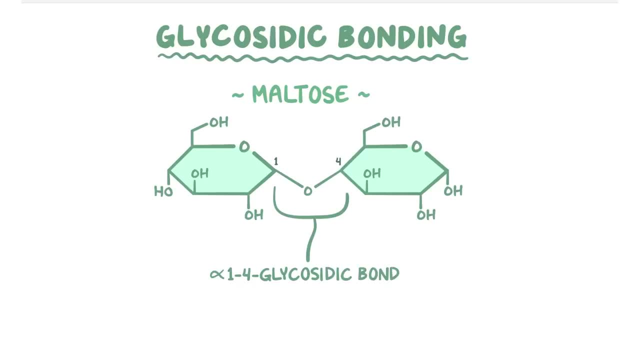 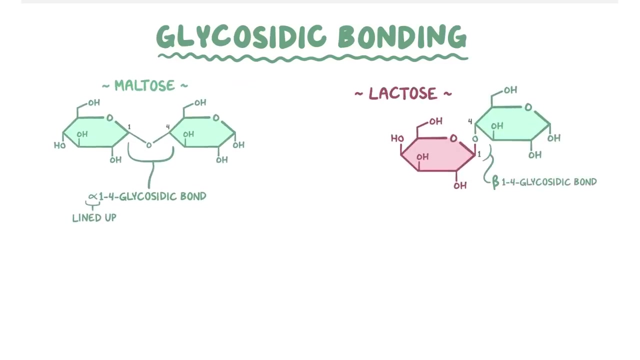 bond between carbon number 1 of one- glucose monosaccharide- and carbon number 4 of the other glucose monosaccharide And alpha, refers to the fact that the molecules are lined up next to each other. Lactose, on the other hand, has a beta 1,4-glycosidic bond, meaning that carbon 1 of galactose and 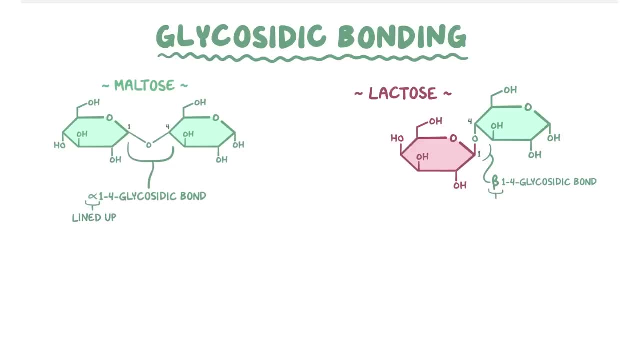 carbon 4 of glucose are bonded, but this time the molecules are stacked, with one higher than the other. Finally, sucrose has an alpha 1,2-glycosidic bond, meaning that carbon 1 of glucose and carbon 2 of fructose are bonded. 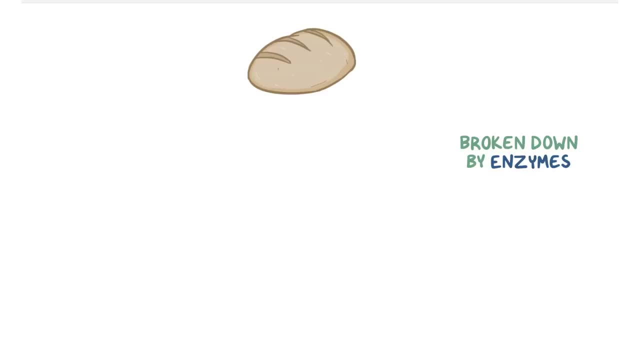 Now, when you eat something like a piece of onion bread, enzymes start breaking down the disaccharides, oligosaccharides and polysaccharides into monosaccharides, so they can be absorbed. Different enzymes help to break down different linkages. 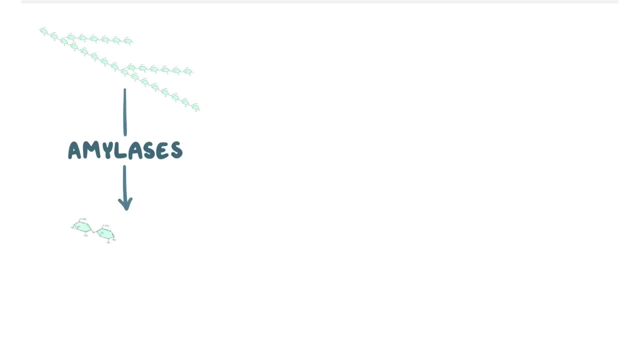 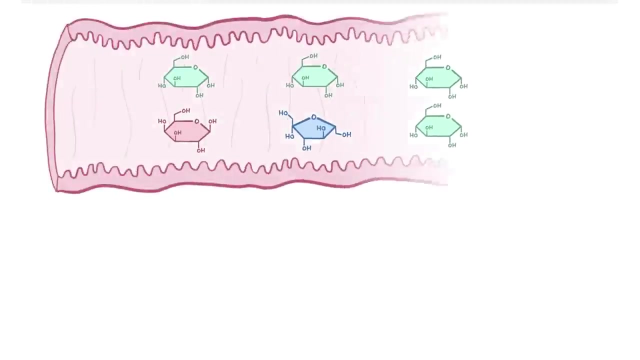 For example, amylases break down large polysaccharides like starch, Whereas lactase sucrase and maltase break down lactose, sucrose and maltose into their monosaccharides, The individual monosaccharides that result from the digestion of larger carbohydrate. 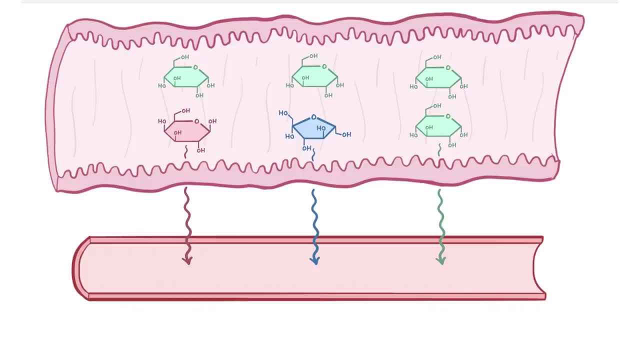 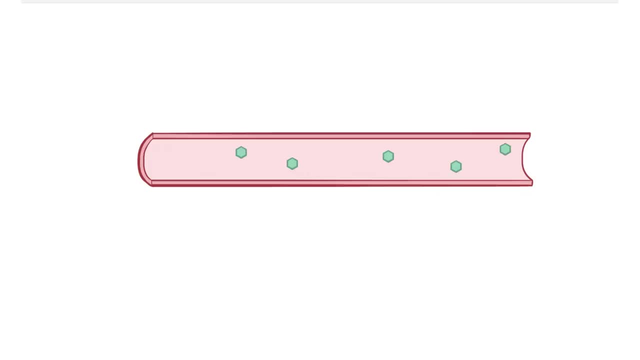 molecules cross the gut lining and get into the bloodstream to get used by the body. When glucose levels in the blood increase after eating, the pancreas releases the hormone insulin And this helps move glucose into all cells for energy. Insulin helps stimulate the liver to store glucose as glycogen in a process called glycogenesis. 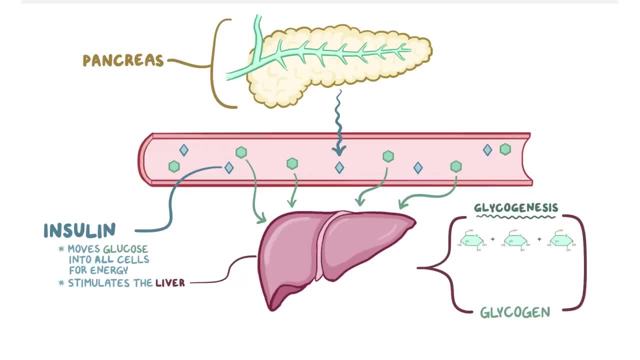 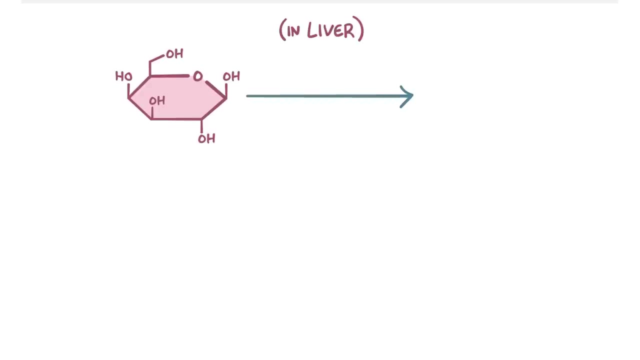 which is when some of the glucose molecules get linked together with alpha 1,4 and alpha 1,6 glycosidic bonds to form a polysaccharide called glycogen. Insulin also promotes fat and protein synthesis. Now metabolism of galactose has an initial step, where an enzyme in the liver converts. 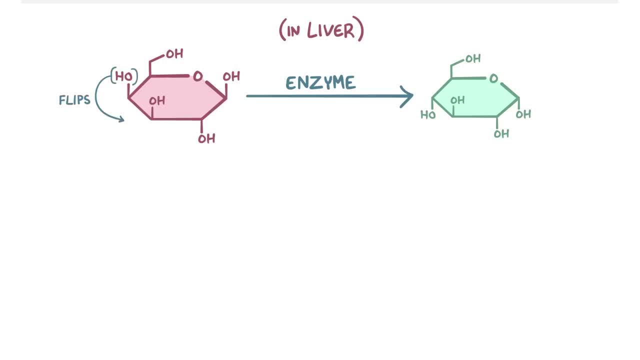 galactose into glucose. It basically flips the orientation of the OH group on the 4th carbon. Just like that, galactose can become just another glucose molecule in the liver. Fructose, though, is handled a bit differently by the liver. 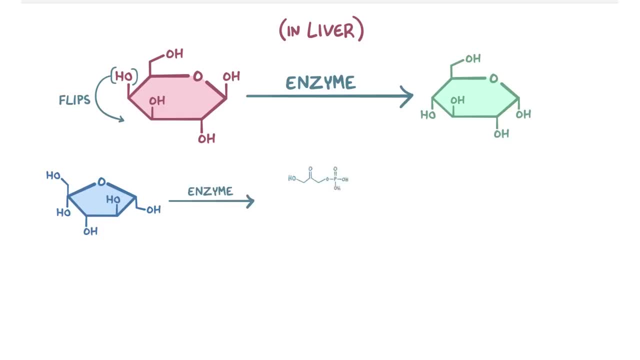 Fructose has a total of 6 carbons and most of it is broken down into two 3-carbon molecules and sent into glycolysis to help generate energy When energy is needed. all three monosaccharides are metabolized through glycolysis. then the 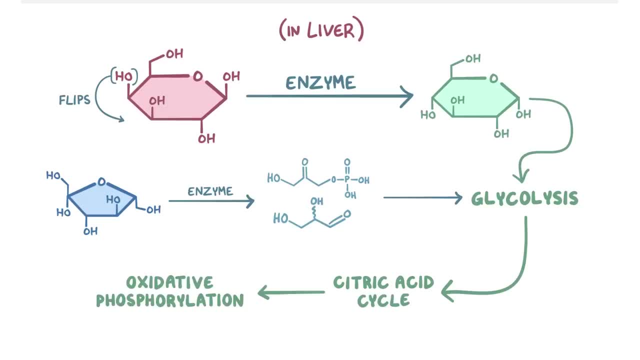 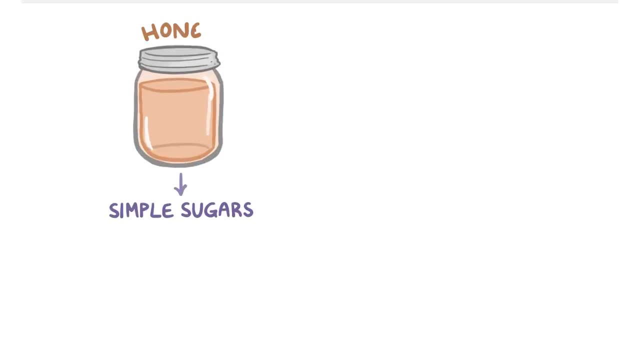 citric acid cycle and oxygen, And that's it. It's a very simple process. Ultimately, all digestible carbohydrates, regardless of whether they come from simple sugars in honey or from starches in baked potatoes, are broken down into their component. 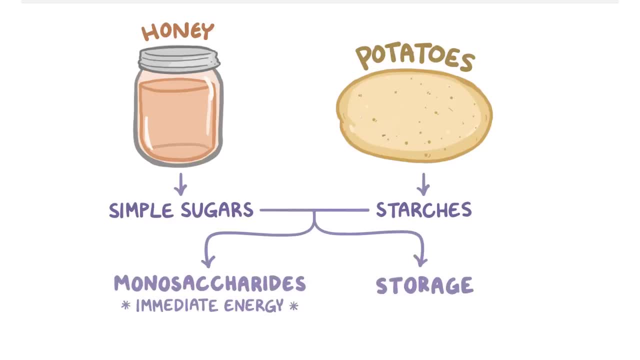 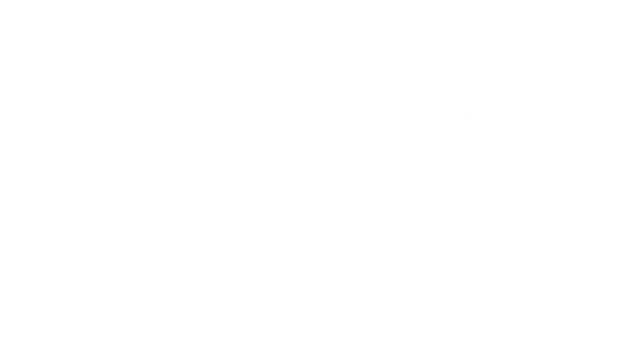 monosaccharides for immediate energy use or stored away for a rainy day, depending on what the body needs. The National Academies of Sciences, Engineering and Medicine recommended that a healthy diet contain 45-65% of its calories from carbohydrates. 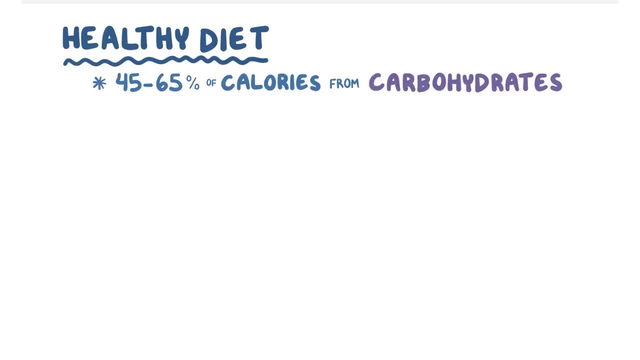 What's the difference? It's a lot. The number of calories you need to maintain your weight depends on things like your age, sex, height, weight and activity level. For example, let's take this slightly active 40-year-old woman who's 5 foot 9 inches. 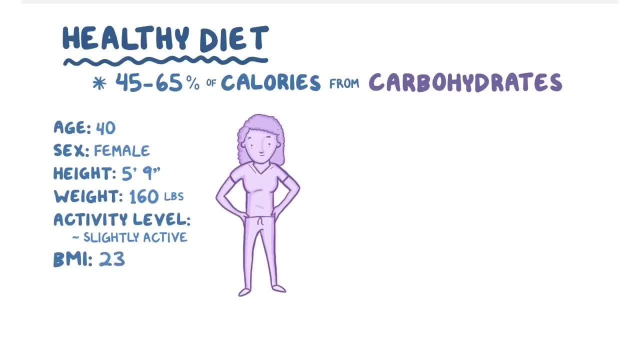 and 160 pounds, with a BMI of 23.6, and requires a 2,000 calorie diet. and let's say she wants to aim for 55% of her calories from carbohydrates. So that's 55% of 2,000 or 1,100 calories. 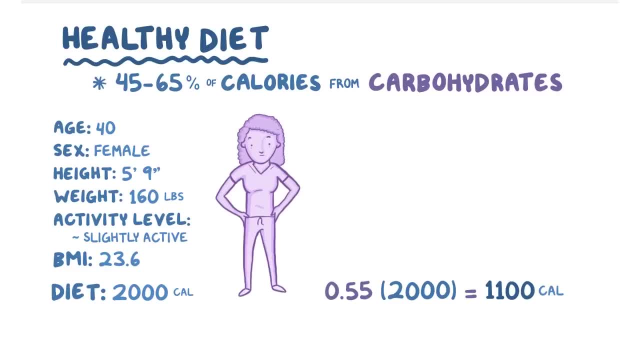 And there are different types of carbohydrates. First there's fiber. The general recommendation is to get 28 grams of fiber in a 2,000 calorie diet With roughly 0 to 2 calories per gram of fiber, that's about 56 calories or about 3% of. 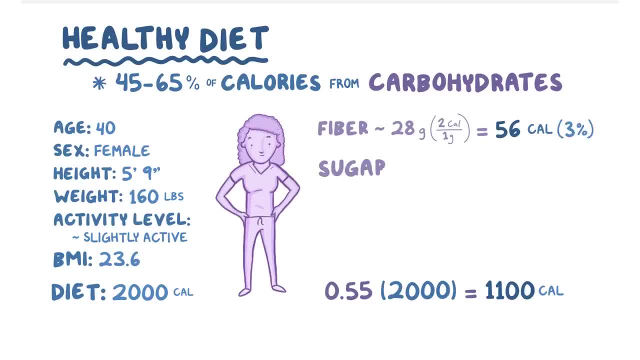 her total calories. Next, there's sugars, both the kind that are added to foods and those naturally found in whole foods. There are a few formal recommendations for total or natural sugar intake. However, updated Canadian nutrition labels are based on a daily value of 100 grams or. 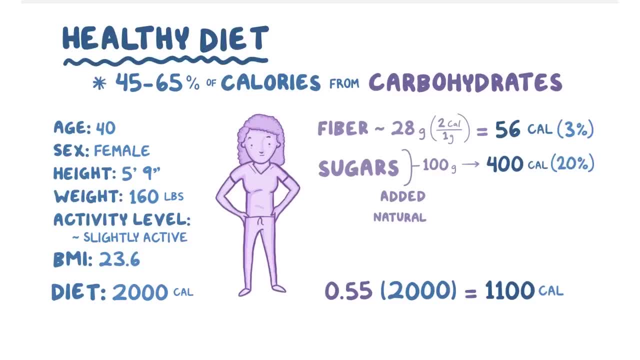 400 calories from total sugars, which is 20% of a 2,000 calorie diet. When it comes to added sugars, both the World Health Organization and the US Dietary Guidelines recommend that they make up fewer than 10% of total calories. 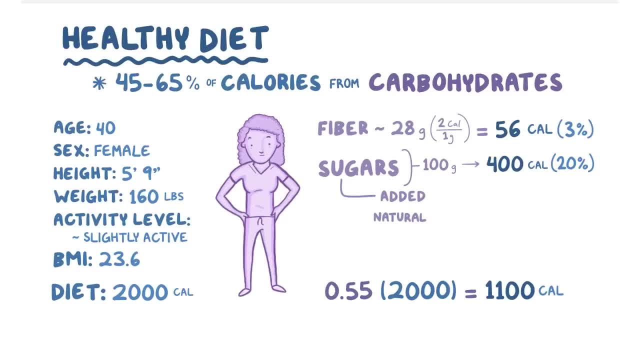 Just like her goal for total carbohydrates, she's aiming for the mid-range of the added sugars recommendation, which would be 100 calories, or 5% of her total calories. So she's aiming for the mid-range of the added sugars recommendation, which would be: 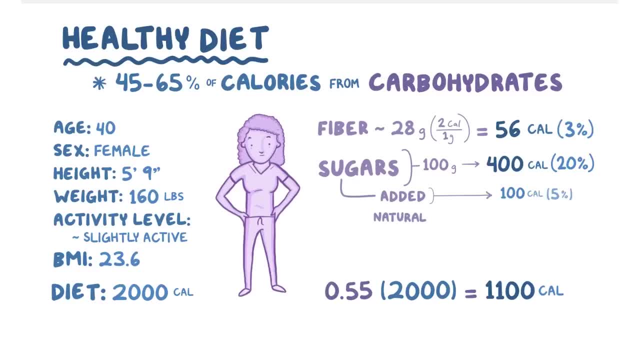 100 calories, or 5% of her total calories. Using this approach, the remainder of her total sugar calories- 300 calories or 75 grams- would come from the sugars found in fruits, vegetables, dairy and grains. This would be 15% of her total calories, and that leaves 640 calories, or 160 grams from. 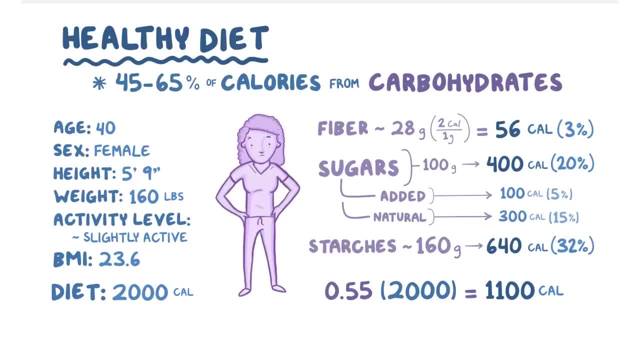 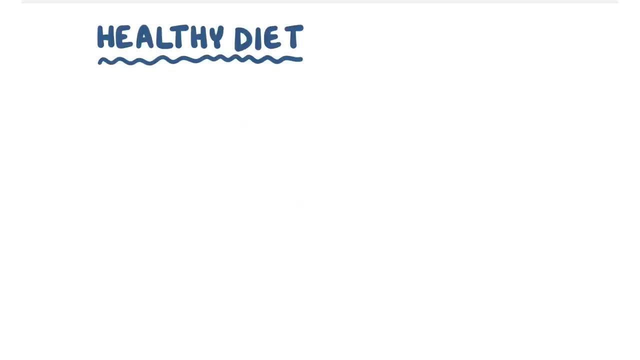 starches, or 32% of her total calories, to reach her carbohydrate intake goal. Now, eating a healthy diet means choosing foods that are as nutrient-rich as possible And foods that contain fiber, starch and natural sugars, like fruits and vegetables. 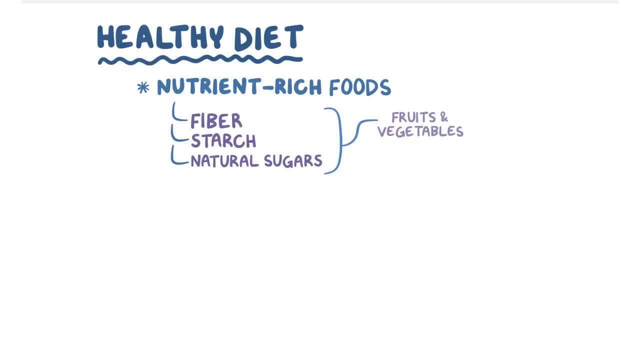 tend to be richer in nutrients than those with added sugars. Having said that, processed and packaged foods are a part of most people's diets, so carefully reading nutrition labels can help you compare foods and choose more nutrient-rich options, Generally speaking, picking foods and beverages that are higher in nutrients, like fiber and 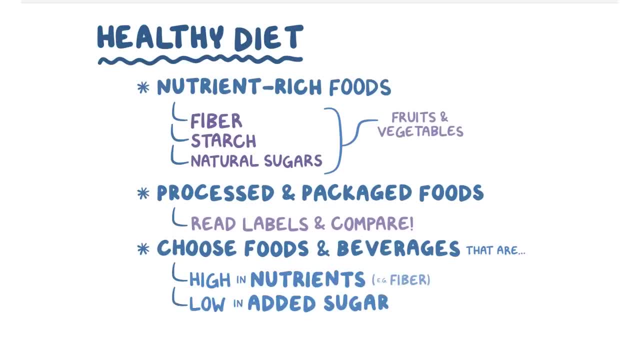 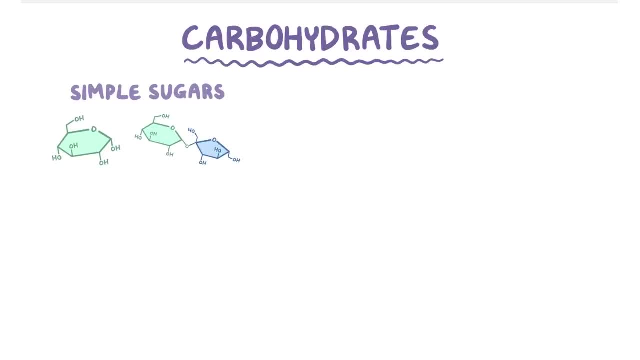 lower in added sugars is best. Alright, as a quick recap, there are various types of carbohydrates. Simple sugars are monosaccharides and disaccharides that the body can readily absorb. Starches are polysaccharides that take longer to absorb.